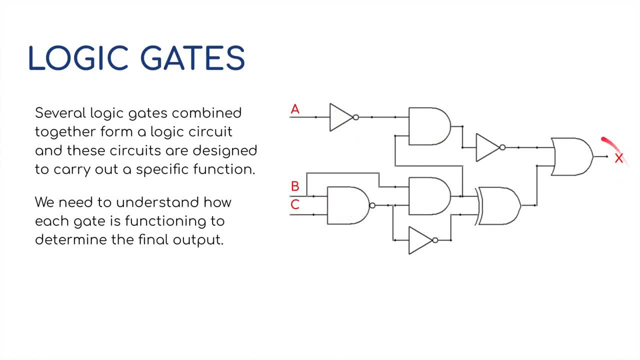 All the electricity is going to pass through this circuit until it gets to the final X here, which is the output. We need to understand how each gate is functioning to determine the final output, what each of these mean. Okay, here we have the NOT gate. 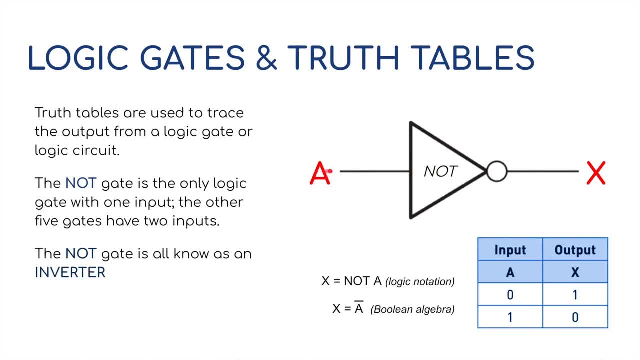 which is also known as the inverter gate. As you can see, we've got one input going into it and then we've got an output going out of it. All the NOT gates- for example, the NOT, the NOR and the NAND- all have one of these little circles in front of the actual gate. 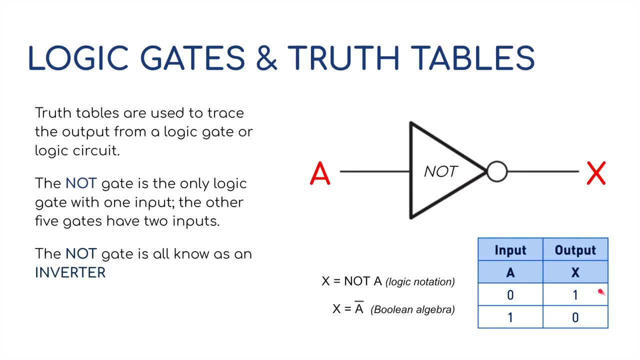 And here is an example of a truth table. Now, truth tables are used to trace out the output from the logic gate or the logic circuit. The NOT gate is the only logic gate that has one input, and the other five gates have two inputs. 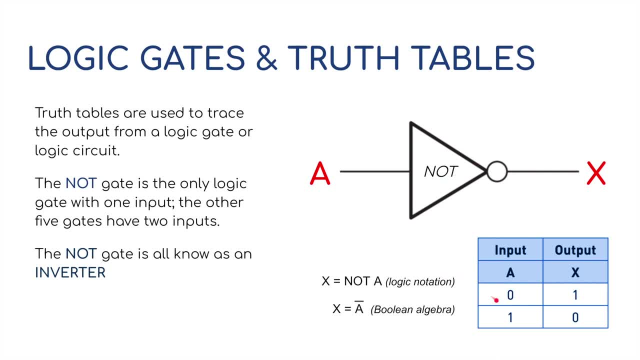 The NOT gate is also known, as I've just said, as the inverter. So, for example, with this one zero going in, If A is set to zero, then the NOT gate will invert it and it will be a one. 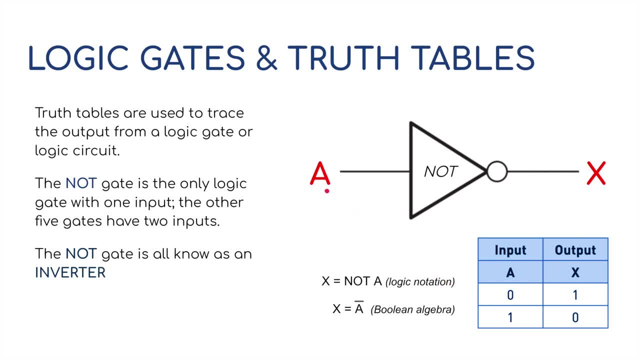 And alternatively, if a one goes in, if A, the input is one, then the output would be zero. In logic notation X is written as NOT A, but in Boolean algebra- and we'll come onto these, I think, in the second or third video- 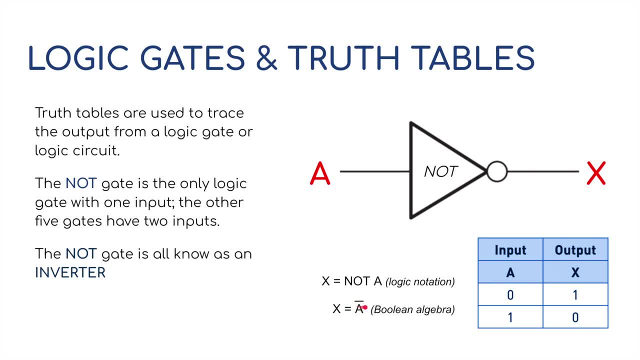 X is seen as A, but with a line over the top of it, which basically means NOT A. It's a little bit like Venn diagrams, in the sense that you've got a line across the top, but in Venn you've got a little line that runs down here. 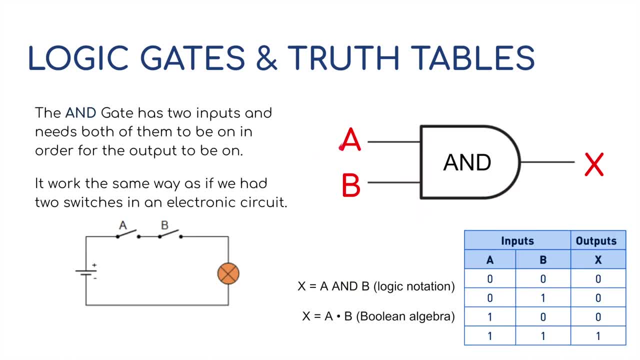 The next gate I want to have a look at is the AND gate, And the AND gate has two inputs, A and B, and need both of them to be on in order for the output to be on as well. It works in a similar way as these switches in series here. 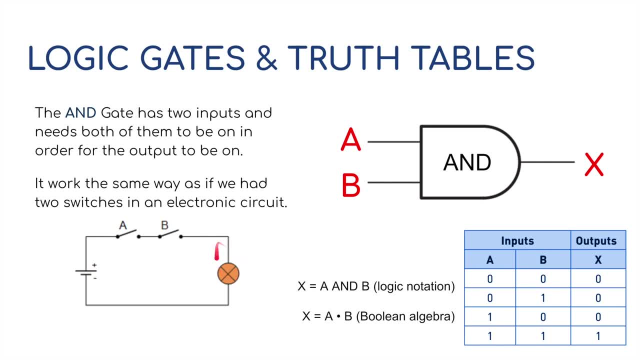 We've got the battery in the circuit and in order to get the light bulb to work, both switch A and switch B have got to be turned on, Obviously, because there's two inputs. the truth table now becomes bigger and we've got four different combinations that could lead to the output. 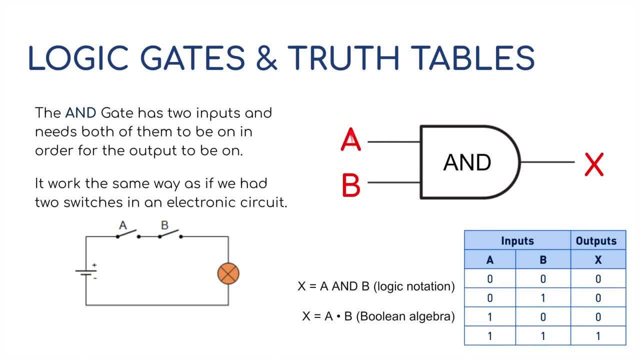 For example, if I put two zeros in here for A and B, then I'll get a zero back out, The same if it's a zero and one, the same if it's a one and a zero. OK, that would lead to this being positive. 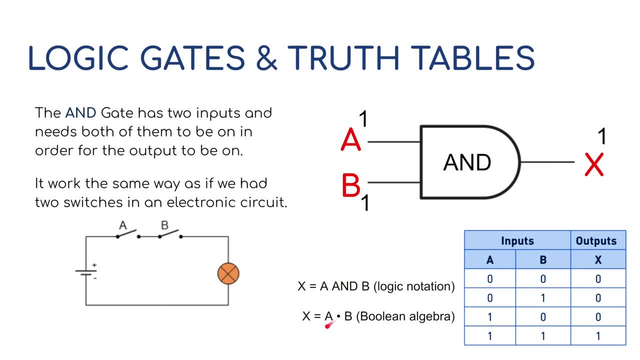 Again Boolean notation A and B, but this time a little bit like Italian or European mathematics, A punto A dot B is seen as being the AND, So not A multiplied by B, but A and B is the Boolean logic expression. 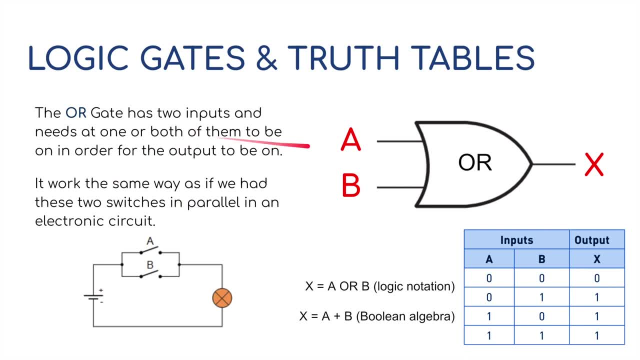 The next gate is the OR gate. Again, the OR gate has two inputs and I've labelled these A and B, But the OR gate works in a different way. One or both of them- one or both A and B- need to be turned on. 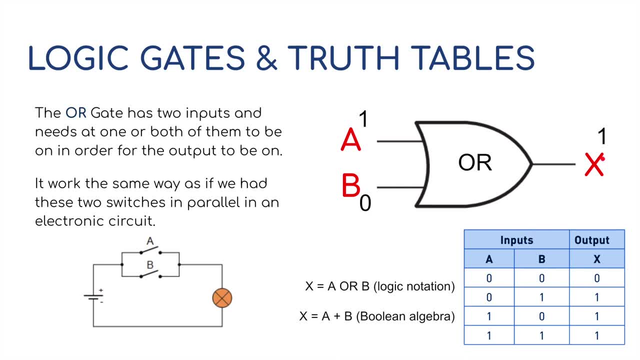 so, for example here, zero and one to be turned on in order for the output to be turned on. Also, with the OR gate, both of them are turned on. A and B are both turned on, as you can see here. then the output will be on as well. 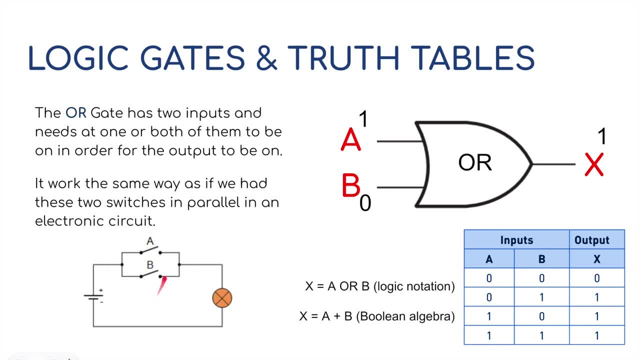 In terms of an electronic circuit, it's similar to switches in parallel. If A is turned on here, look, the bulb would still light up. or if B is turned on, the bulb would still light up. or if both of them are turned on, the bulb would still light up. 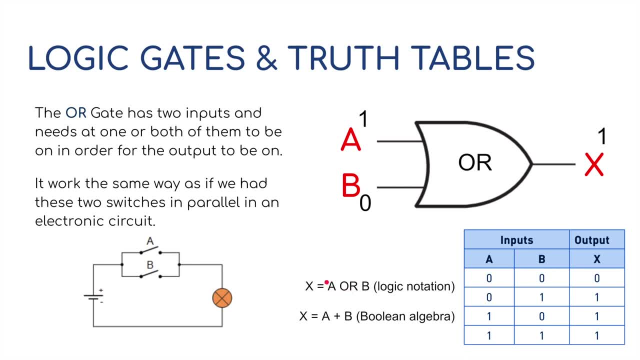 Now this is a bit strange as well, because obviously X equals A or B, but in Boolean algebra, written as an expression, it's A plus B, which is bizarre because you'd think A plus B would be the AND gate. 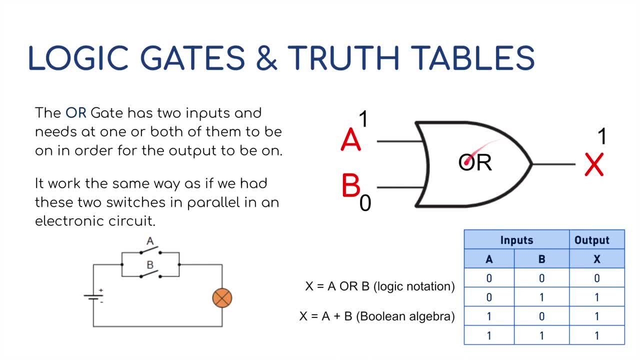 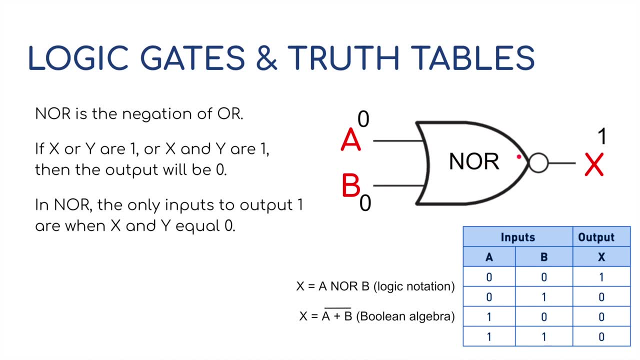 but no. A plus B is the OR gate. Now, the opposite of the OR gate is the NOR gate and, as I mentioned for the first one, the NOT gate. it has one of these little round things on the front of it. 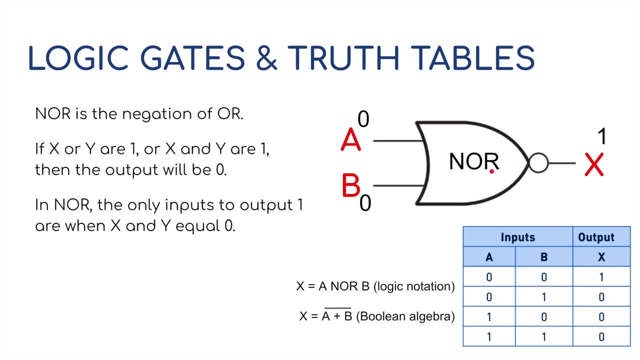 and that means NOT, so, NOT, OR, basically So. NOR is an expression and NOR is an allegation of the OR. So if X or Y are 1, and X and Y are 1,, then the output will be 0. 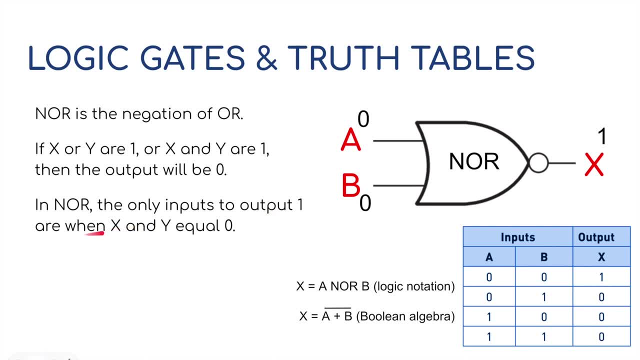 In NOR, the only input to output 1 are when both X and Y equal 0, and you can see that here. So 0, 0 equals 1.. The rest of them, the rest of the combinations, would lead to a 0 output. 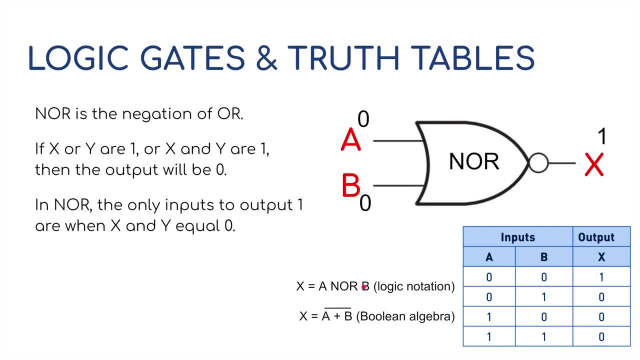 Obviously logic notation A NOR B. but here we've got the same as an OR, gate A plus B, but it's NOT OR, so it has the line over the top of it like this: OK, That's a Boolean algebra expression. 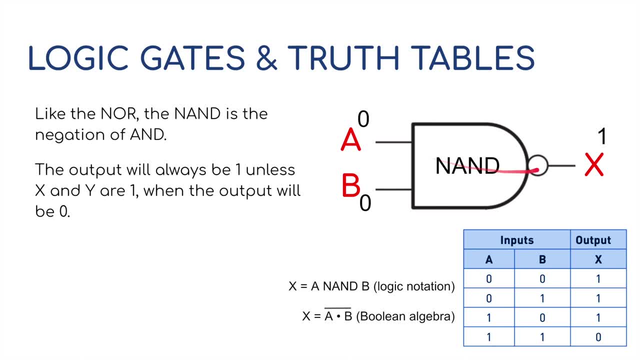 And the same with the NAND gate. It's the negation of the AND It's got one of these round things on the front of it again. The output will always be 1, unless X and Y are 1, when the output will be 0.. 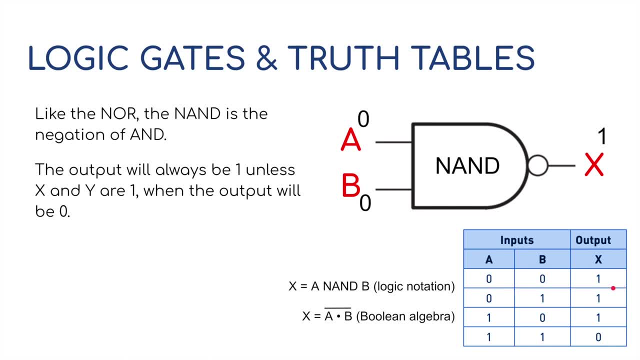 So here we go. So 0, 0 leads to a 1.. 0 and 1 leads to a 1.. 1 and 0 leads to a 1.. But both being on the opposite. the negation of AND would lead to 0.. 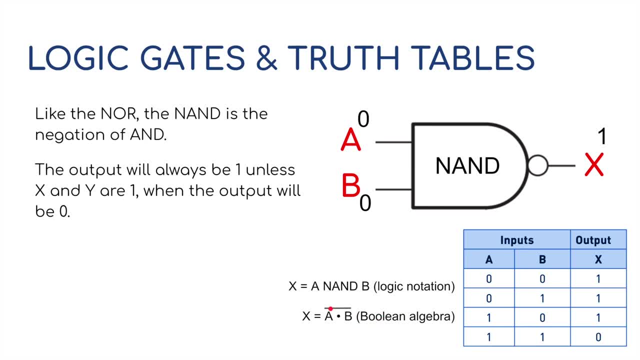 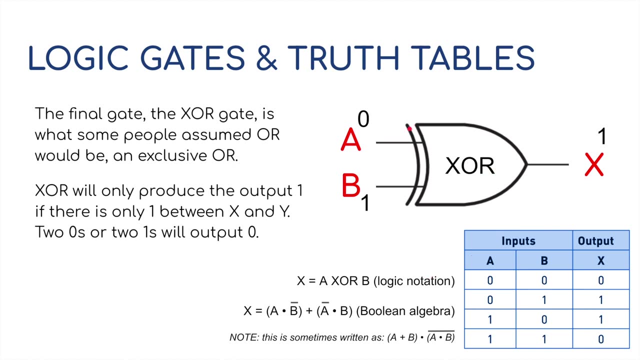 And, as before with the NOR gate, it's A and B, but with the line over the top to specify that it is NOT A and B. OK, And then finally, we've got one called an X OR gate, And it's basically an OR gate with this line. 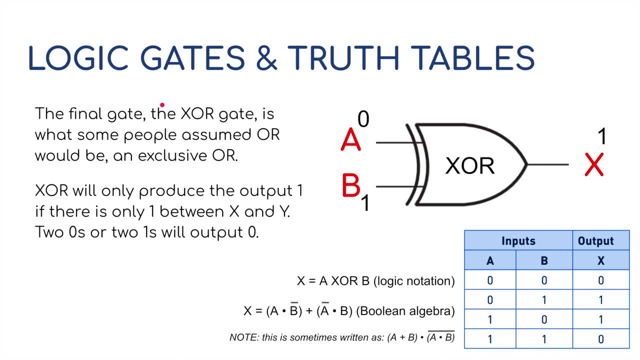 around the back of it. The final gate, the X OR gate, is what some people assume. the OR gate would be An exclusive OR. But what does that mean? Well, X OR will produce the output 1 if there is only 1 between X and Y. 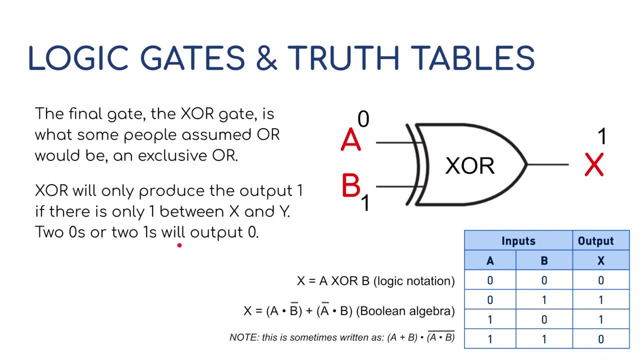 Two 0s or two 1s will output a 0. So, as you can see here it's what they call an exclusive OR gate. So 0 and 1 works, 1 and 0 works, But if we've got them both on, 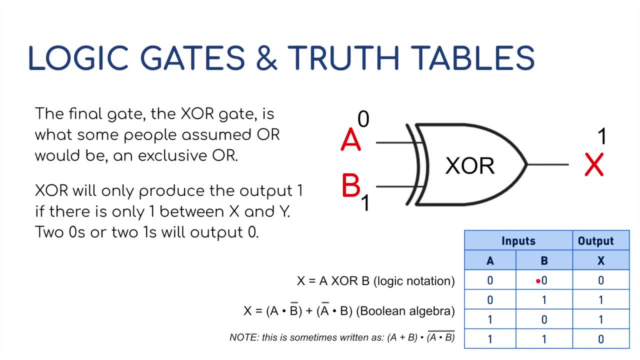 then it would lead to a 0. And again, like the OR gate, two 0s would equal a 0. So logic notation nice and easy: A, X OR B. But in terms of Boolean algebra you've got quite a big statement here going on. 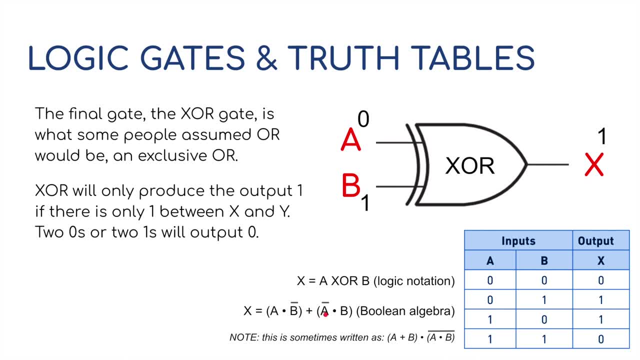 You've got A AND NOT B OR NOT A AND B. It's sometimes written to make it a little bit easier: A OR B AND NOT A AND B, So a little bit confusing, but that is the final gate that we'll be using. 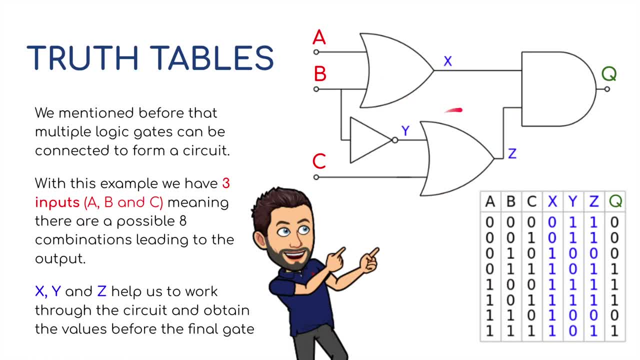 So here I am and we've got a circuit here with four different gates. Well, two of the same, We've got two OR gates, we've got a NOT gate and we've got an AND gate at the end, And we've got three inputs. 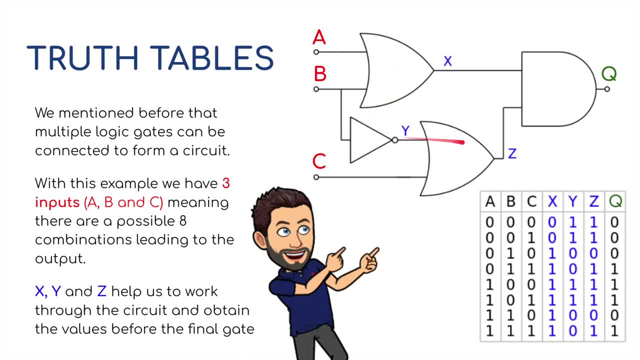 So we mentioned before that multiple logic gates can connect to form a logic circuit. as you can see here The example, we've got three inputs: A, B and C, meaning there are eight possible combinations, Eight combinations of 0s and 1s. 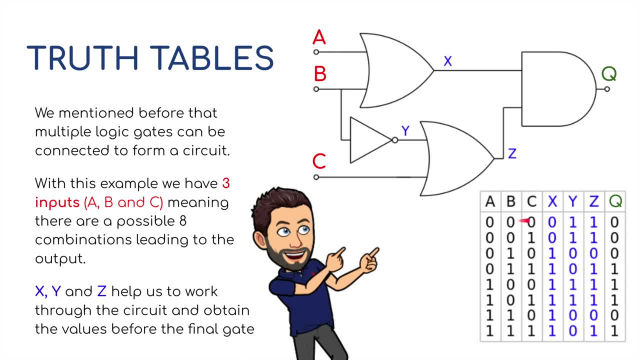 So A, B and C could all be turned on. could all be turned off, sorry, or all be turned on and then anywhere in between. So we've got A in the second one. A is off, B is off, but C is on. 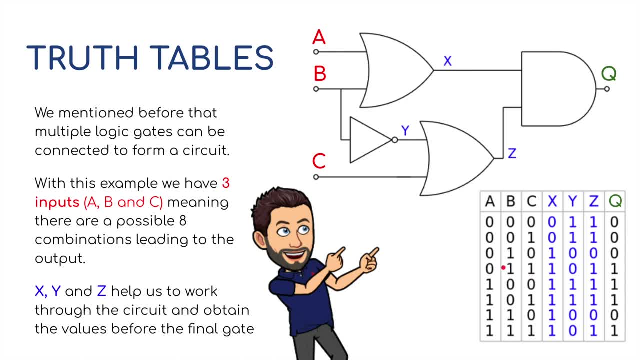 And down here, B and C are on, but A is off. The X, the Y and the Z just make life a little bit easier. When we're working through these- and you will do later on in this chapter- you'll be given a circuit that has to say: 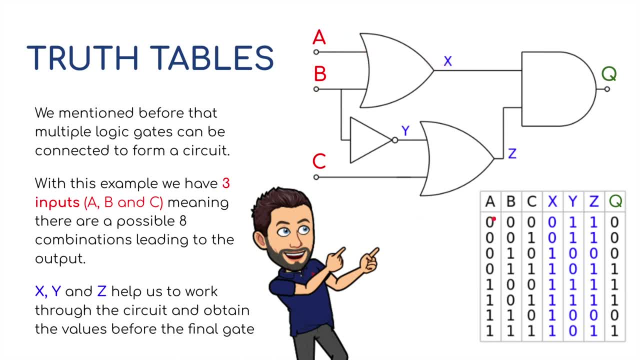 what is the value of Q based on your inputs, and you'll have to create a truth table. So what I've done here is I've put an X after this OR gate, I've put a Y after this- NOT gate- and then a Z after this OR gate. here. 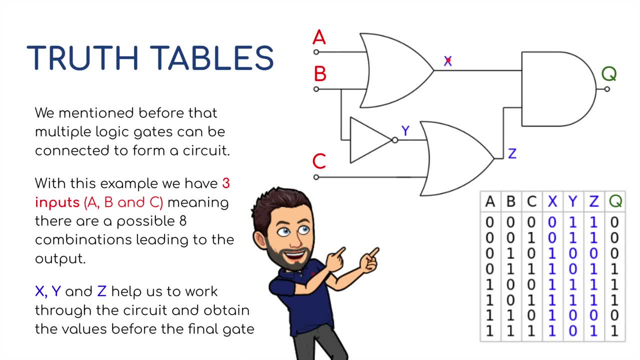 So what I need to do is look at the value for X and the value of Z, so these two here, and that will determine what is going on with the AND gate. So, for example, X is turned off when it goes through here. 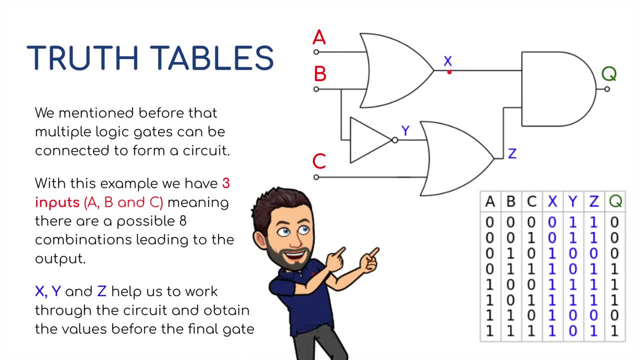 because they're all turned off. so X is off there. so a 0 is going into the AND gate. so we can see that it's going to be 0 despite Z being on. So the only time is when both with the AND gate. 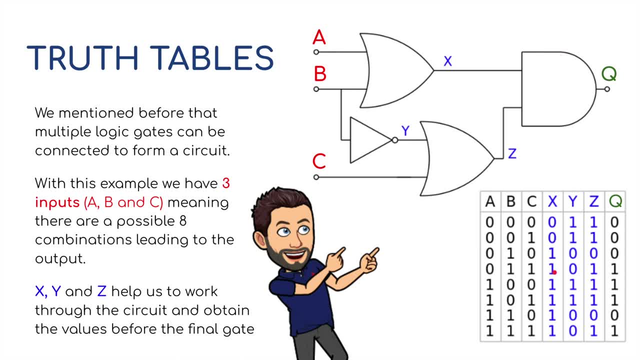 when they're both on. so we're looking down here at the X value being on and the Z value being on, and the same throughout these and this one here. So we've created a circuit which gives us quite a strange looking truth table.